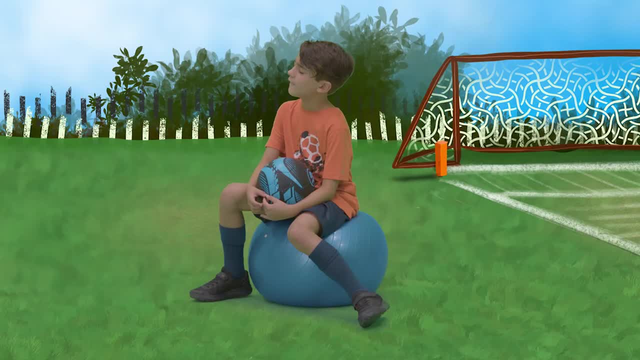 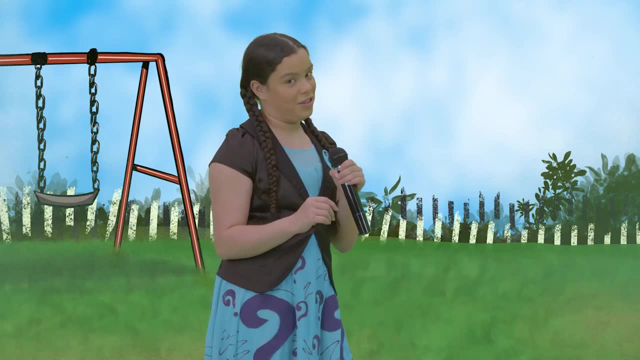 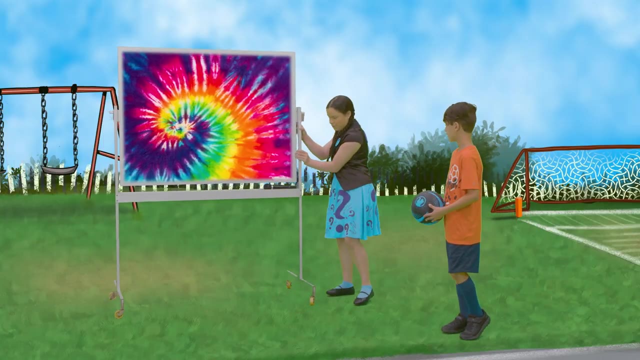 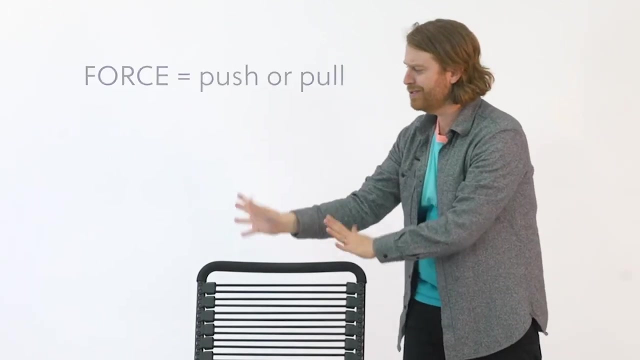 and two. what type of motion is happening? Force in motion, What's that? Let's see if the Gregory Brothers can help explain force in motion. They're a lot of fun, Hi. Force is either a push or a pull, And any movement anywhere starts with a force. 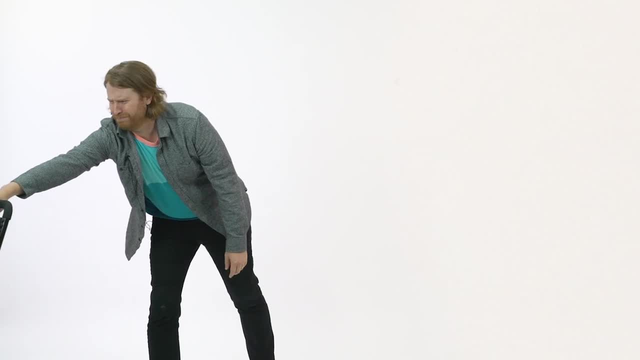 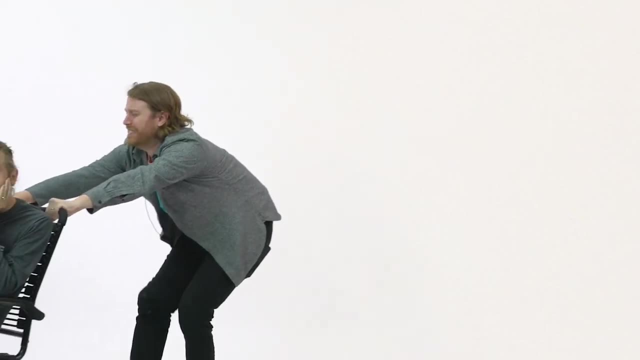 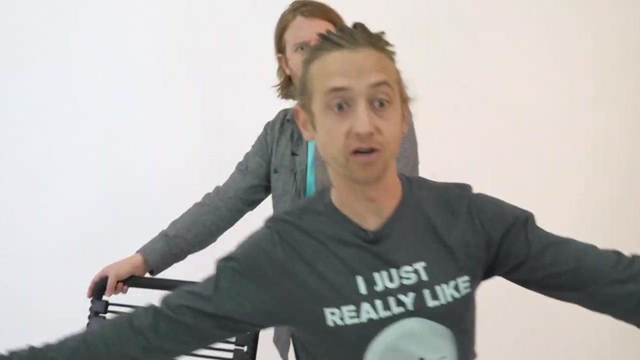 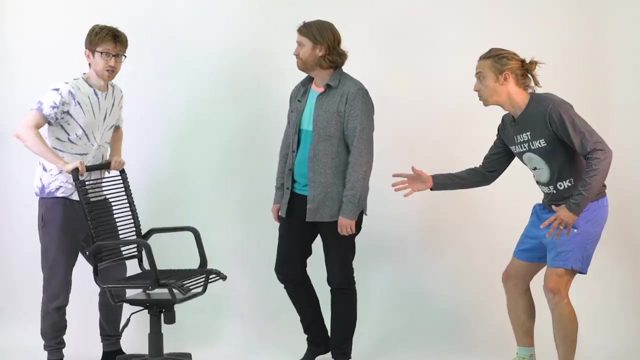 Like when I push this chair Or when I pull it. When I push it Or when I pull it, Motion is movement from one place to another. Motion can be fast Or slow, Motion can stop And motion can change Direction. 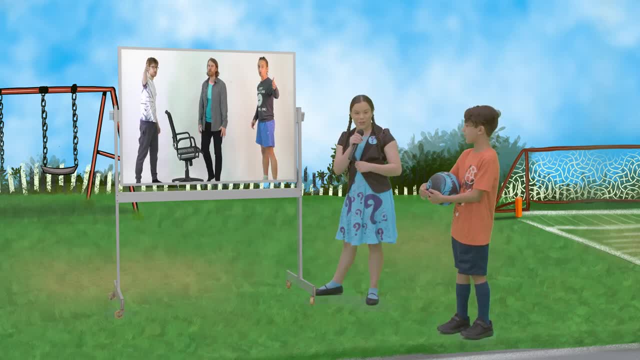 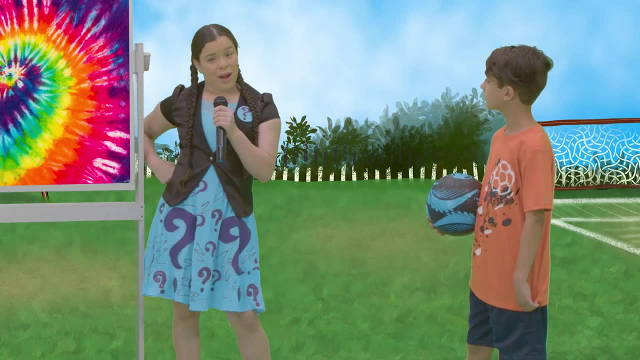 And with force in motion, you can explain How Things Move. So the question for today's game show is: what type of force and what type of motion is happening when this soccer ball gets kicked into the goal? Hurrah the clip. 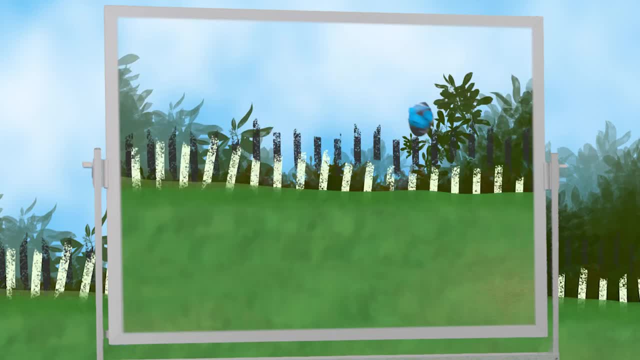 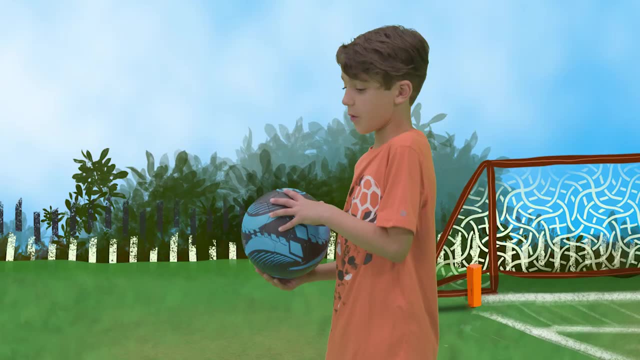 Is the force of a kick, a push or a pull? Is the motion of the ball fast or slow? Does it stop? Does it change? Does it change direction? Oh well, I mean so the ball's kicked And then you know, it goes there. 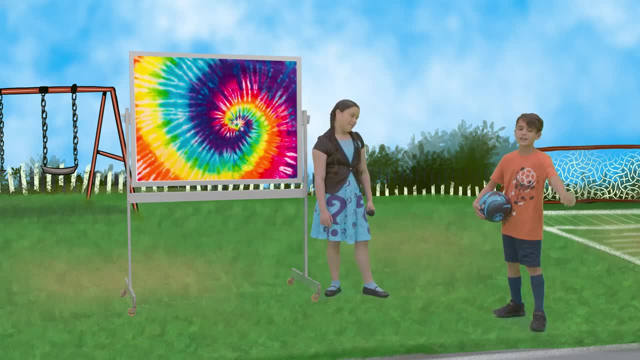 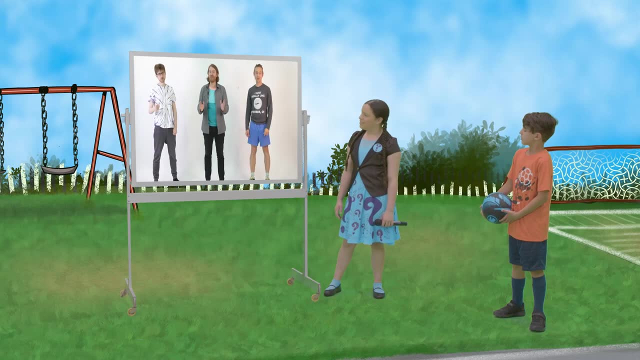 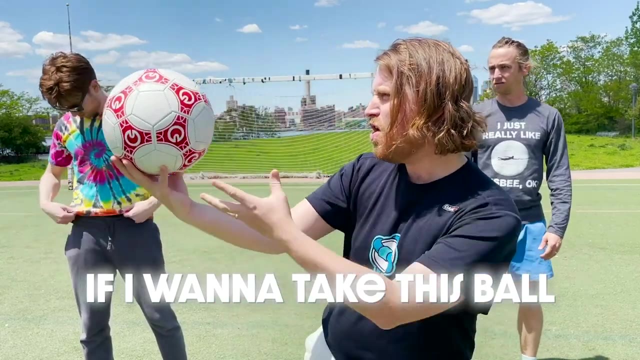 And I could really use some help. We can help. We even have a song And a dance To help you figure out how things move. Sing a dance with us If I wanna take this ball And put it into the goal I got to use. 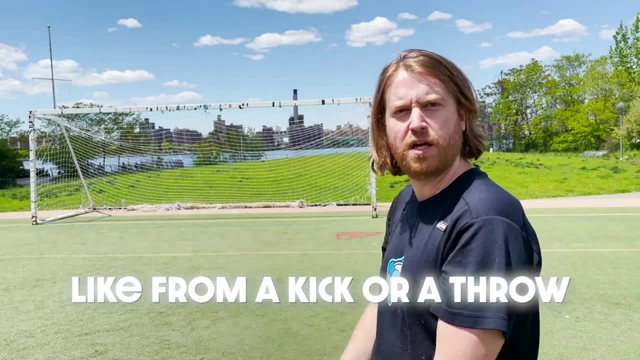 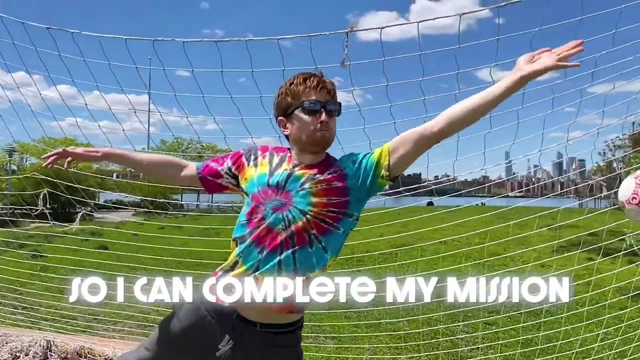 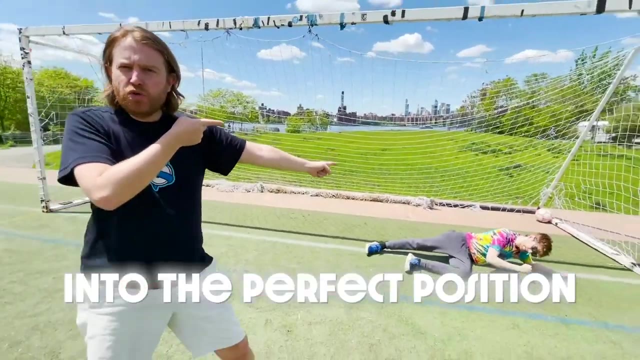 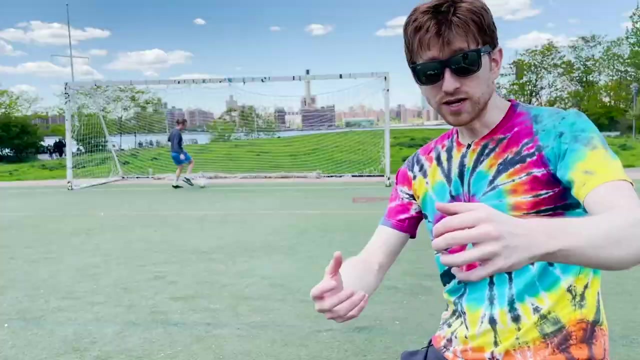 The exact right force, Like from a kick or a throw Force can put it into motion So I can complete my mission Of putting that ball Into the perfect position. Remember, force is any kind of push Or any kind of pull, And when something moves, That's motion. 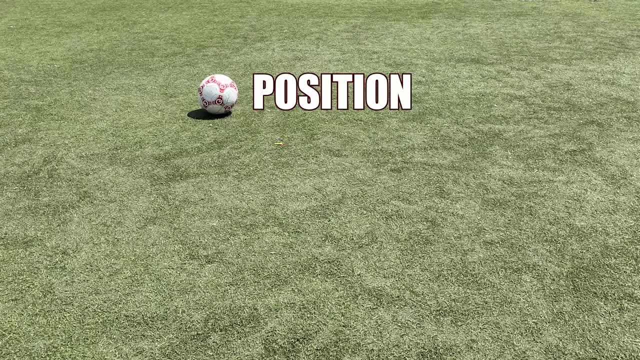 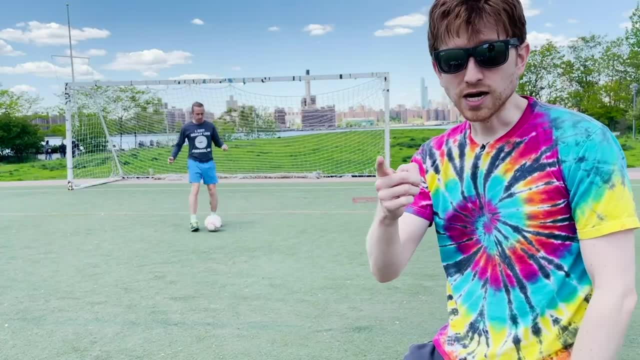 And position. That's wherever the object is, As it's moving And when it stops, Let's use force to put our bodies into motion. However you want, I'm gonna do a push And pull my arms And twist my legs When I count down from four. 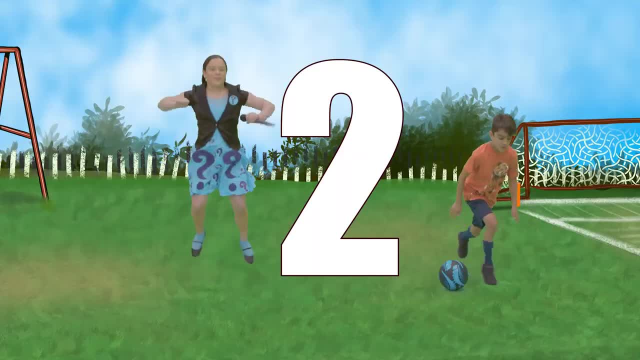 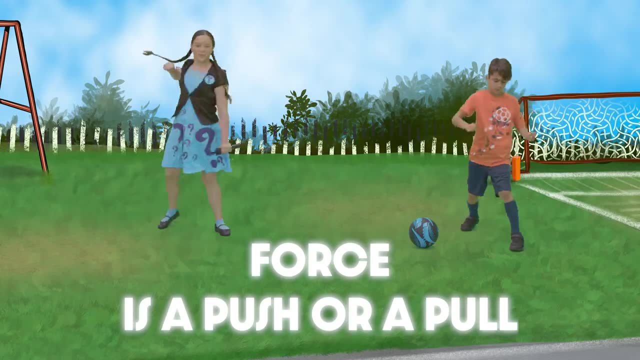 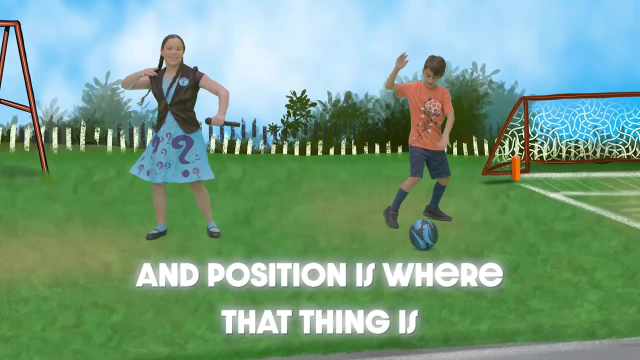 Let's freeze our bodies in one position: Four, three, two. one freeze Force is a push or a pull. When an object moves, That's motion And position is Where that thing is At any given moment. So if you wonder why, 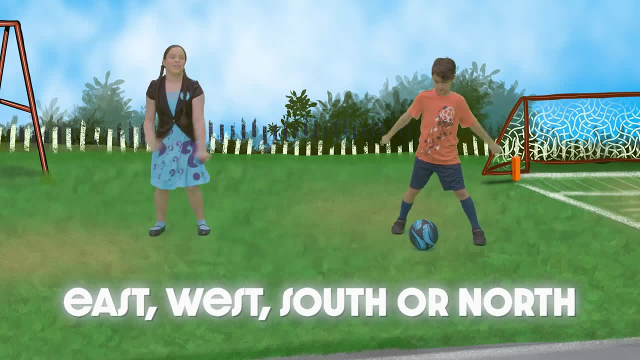 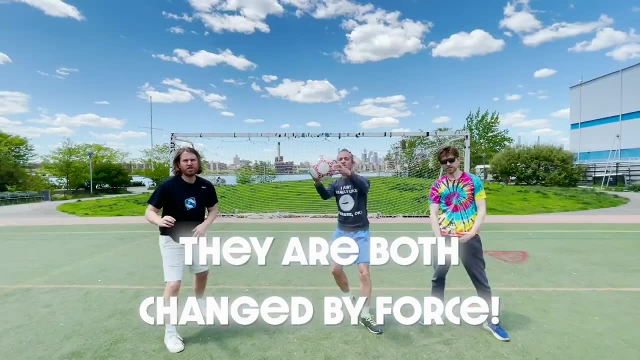 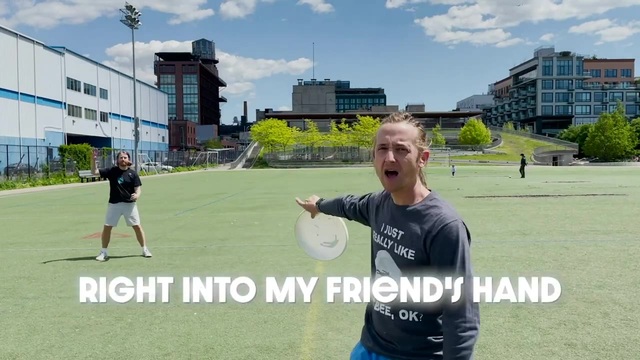 An object is moving East, west, south or north. It's cause motion and position. Yeah, they are both changed by force. If I wanna throw this frisbee Right into my face Or into a friend's hand, I got to use the exact right force. 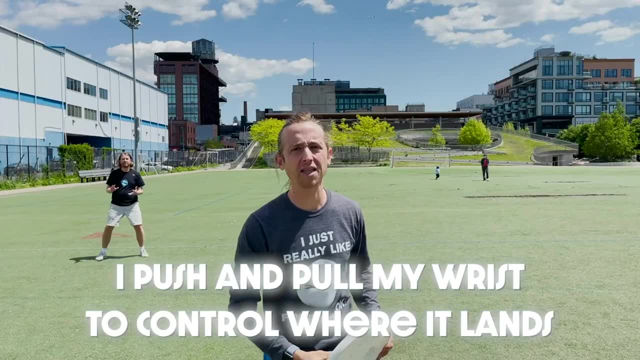 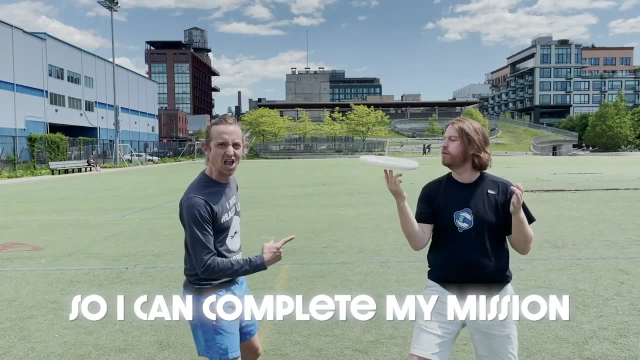 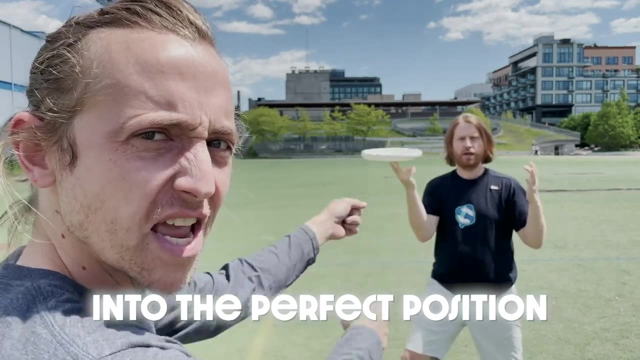 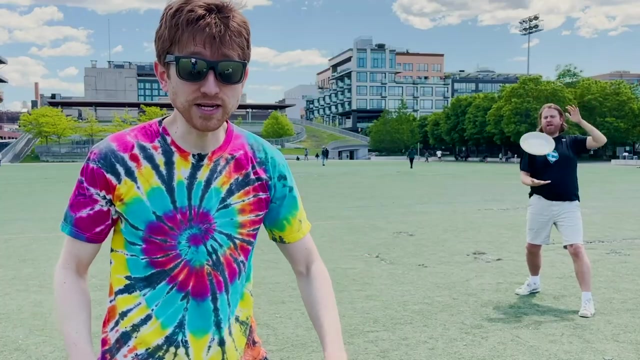 I push and pull my wrist To control where it lands. That force puts it into motion So I can complete my mission Of putting my flying frisbee Into the perfect position. Dance break: Let's put our bodies back into motion, using force Dance to change the position of your arms and legs. 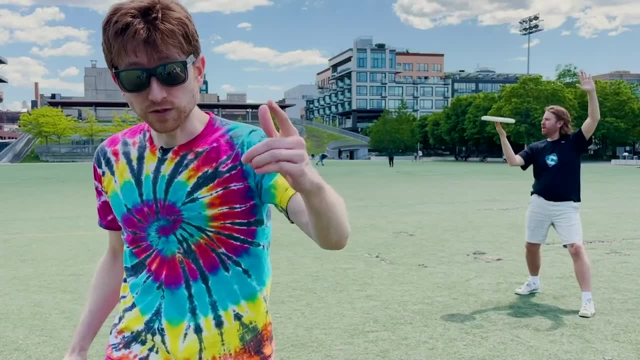 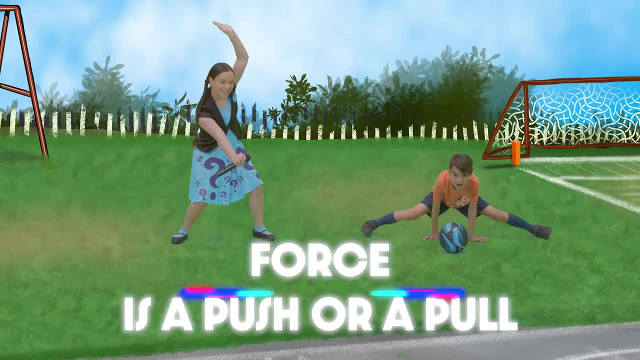 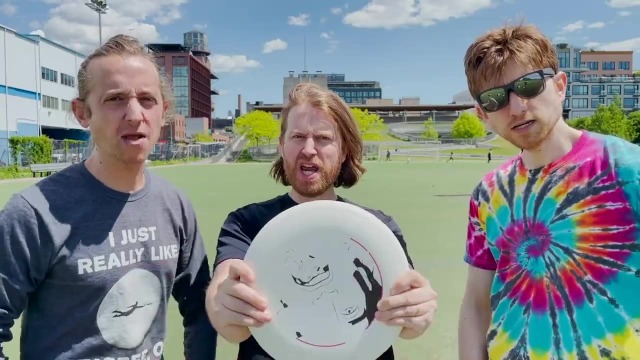 Any way you want. And when I count down from four, Let's freeze our body in one position. Four, three, two, one freeze Force is a push or a pull When an object moves, That's motion And position is Where that thing is. 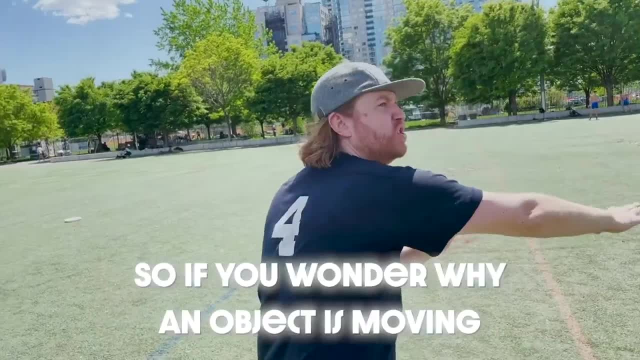 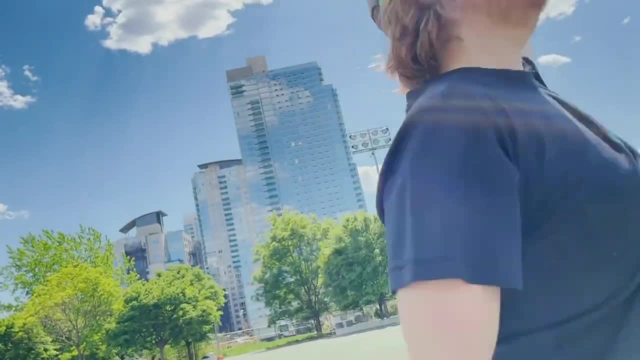 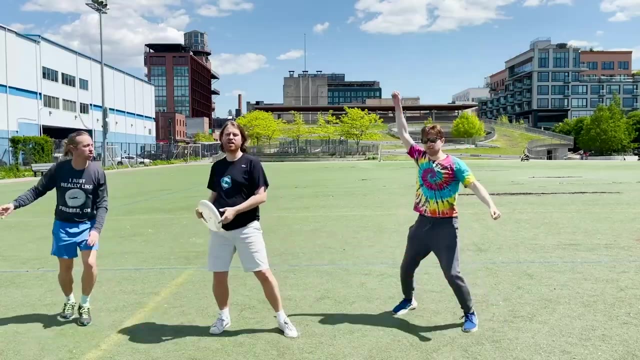 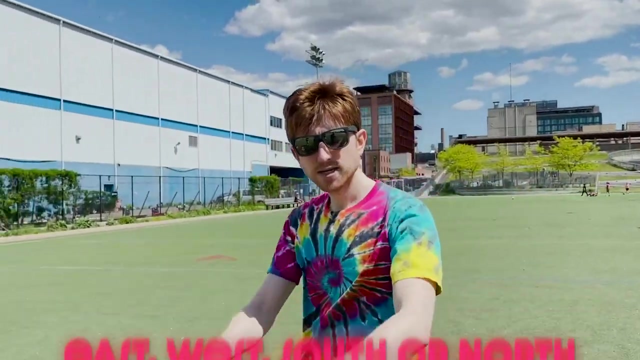 At any given moment. So if you wonder why An object is moving East, west, south or north, It's cause motion and position. Yeah, they are both changed by force. Yeah, if you wonder why An object is moving East, west, south or north, 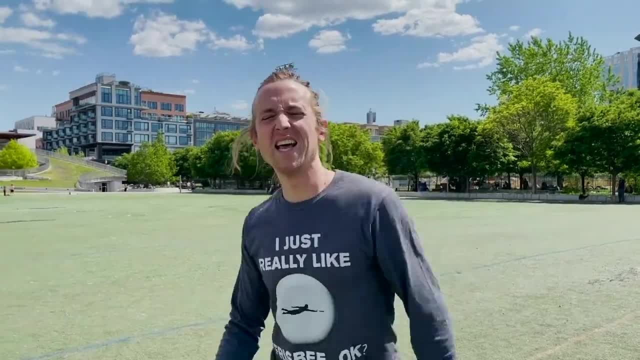 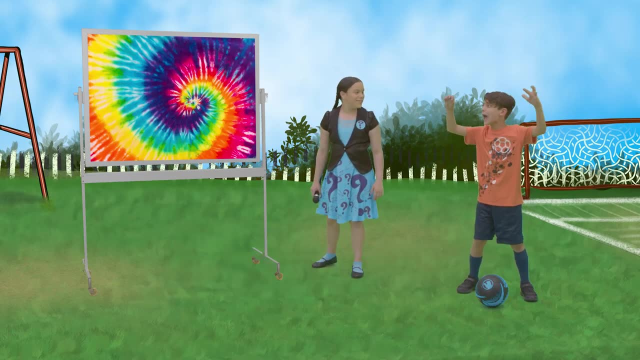 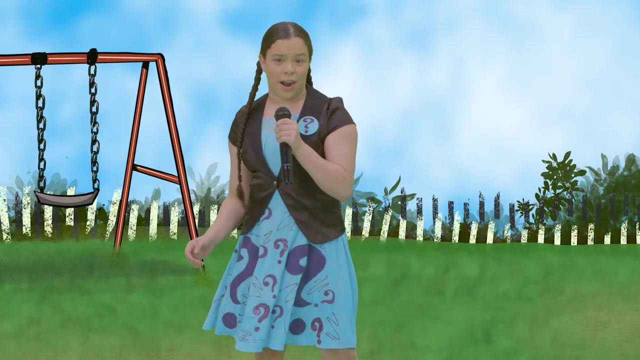 It's cause, motion and position. They are both changed by force. That was epic. I knew they'd get things moving. Alright, viewers, it's time to take out your game cards And write down your answer to what type of force And what type of motion is happening. 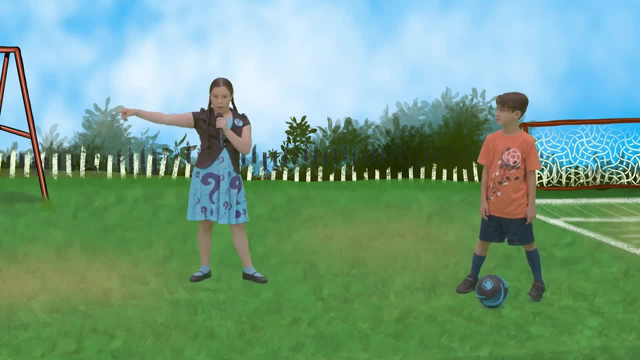 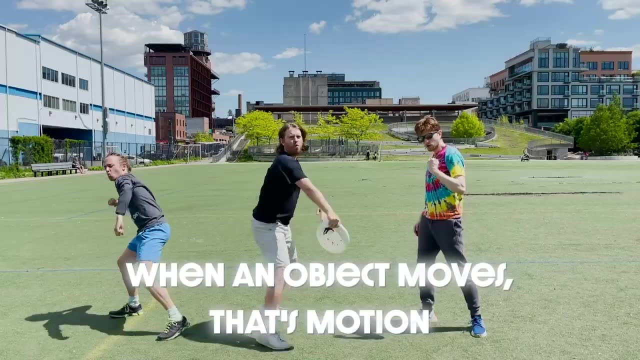 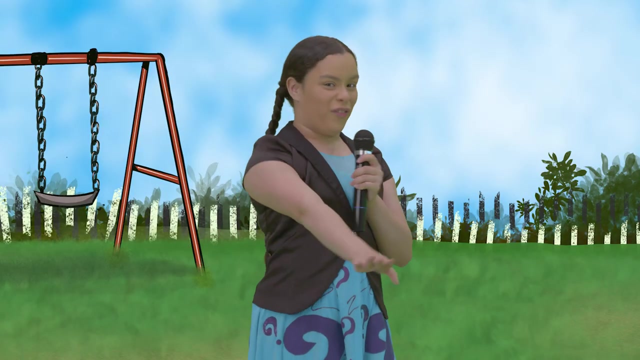 When this soccer ball gets kicked into the goal. If you get confused, just go back and sing the song again. Force is a push or a pull. When an object moves, That's motion. Get ready to pause the video, Because when we come back we'll reveal the answer. 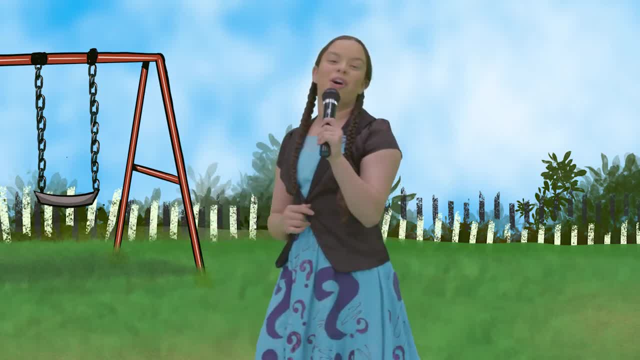 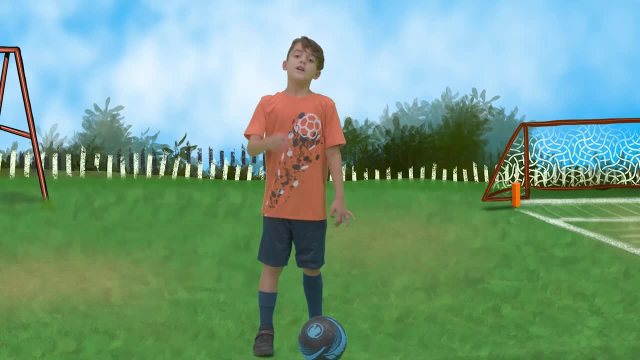 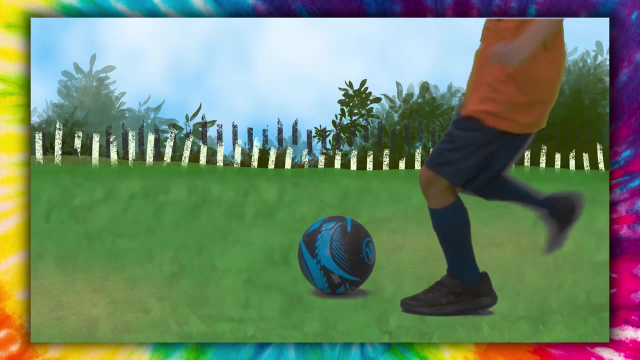 And we're back with How Things Move. Did you figure out the force and motion of the soccer ball being kicked? I think I got it. Did you For kicking the soccer ball? I said the force was a push Because my foot pushed the soccer ball forward. 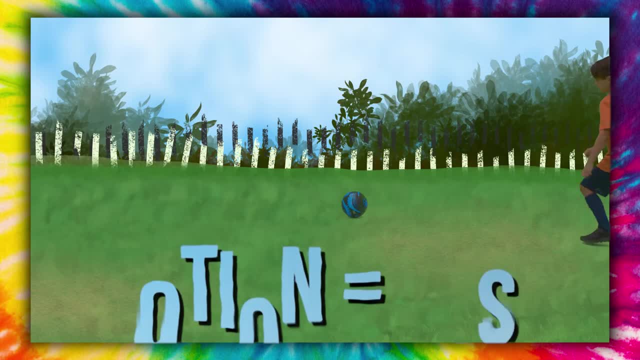 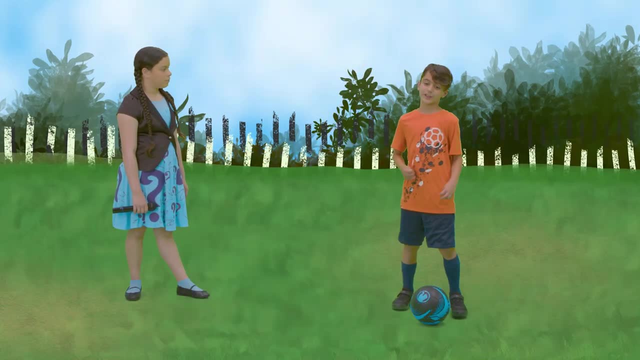 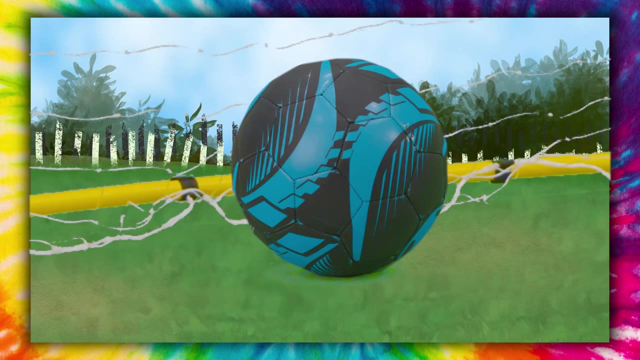 Away from me For motion. I said it moved fast Because I kicked the soccer ball With a strong push force. The stronger the force of the kick, The faster the motion of the ball. Then the motion of the ball stopped When it landed in the net. Guess what? 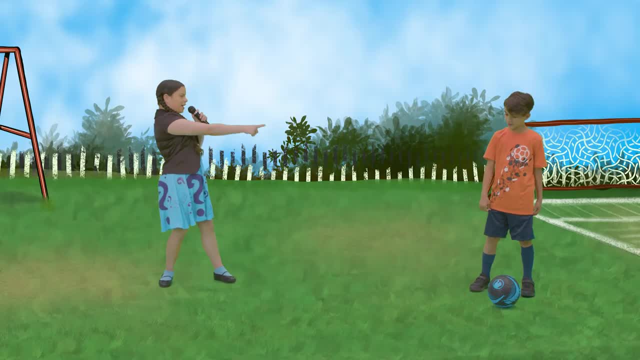 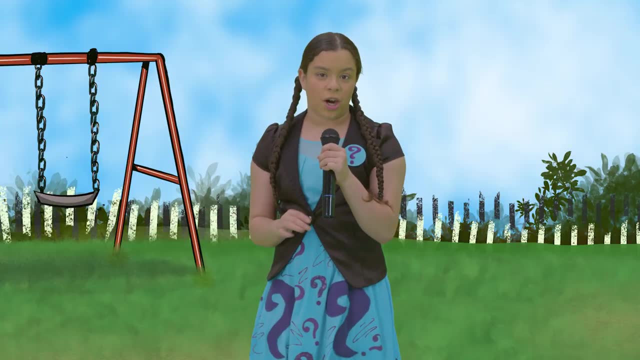 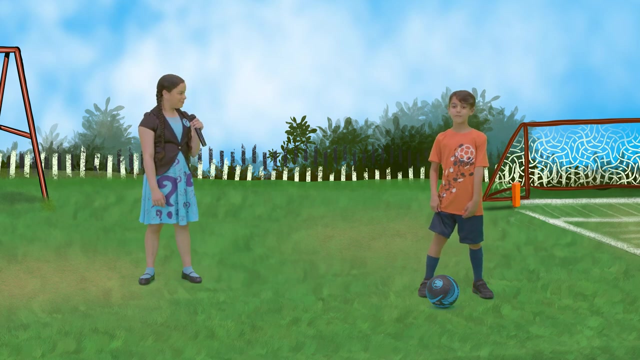 If you got the same answer as Rick Ricardo. You know How Things Move. For a bonus On your game card, Write down another object in motion. you see And write down its force in motion. Alright, Who's up for a game of force in motion? 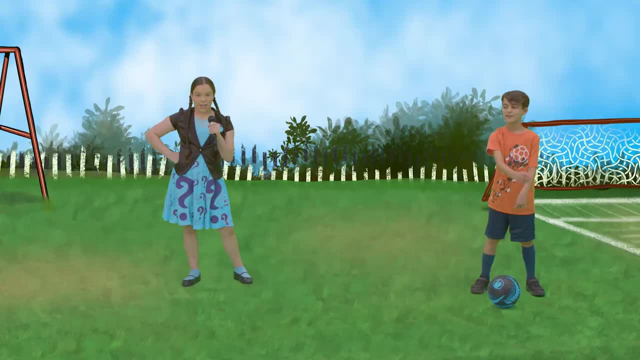 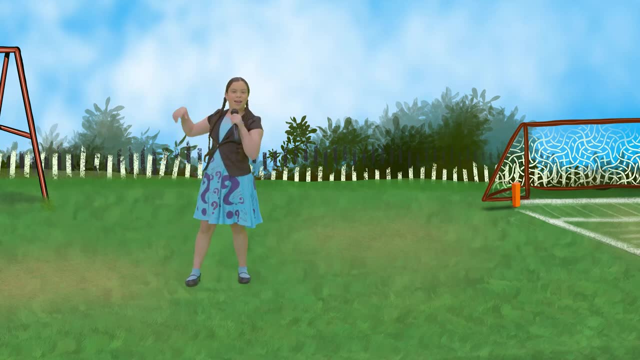 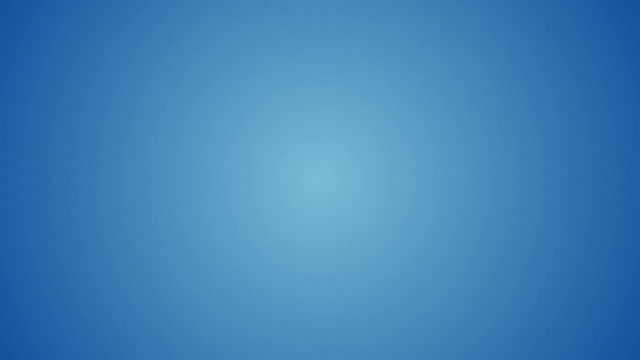 I mean A game of soccer. Have fun. I'm Ms Grouchy Holding it down on the playground. We'll see you next time. on How Things Move, Force is a push or a pull. When an object moves, that's motion, And position is where that thing is. 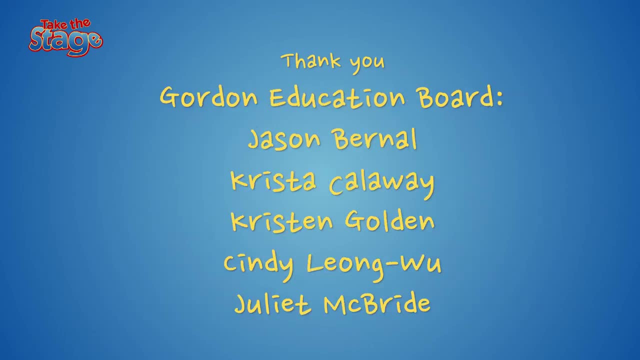 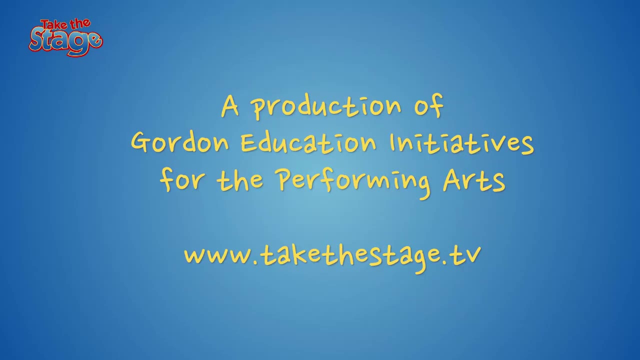 At any given moment. So if you wonder why an object is moving East, west, south or north, It's cause motion and position. Yeah, they are both changed by force.